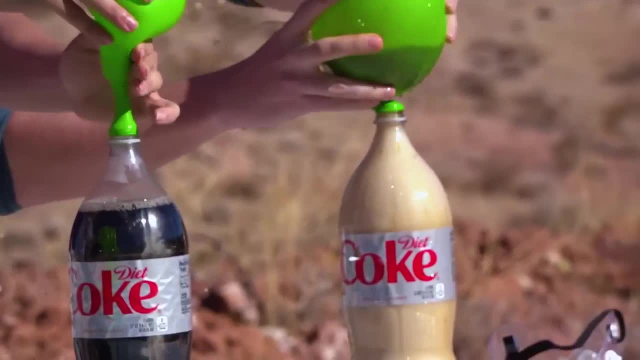 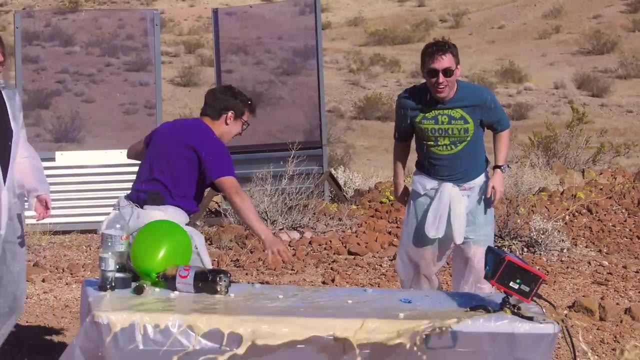 Oh my God, no. So we're just going to like drop them, Squeeze the line down in there. It's going to Oh oh oh, Grenade. Well, yours kind of survived. That's pretty cool. 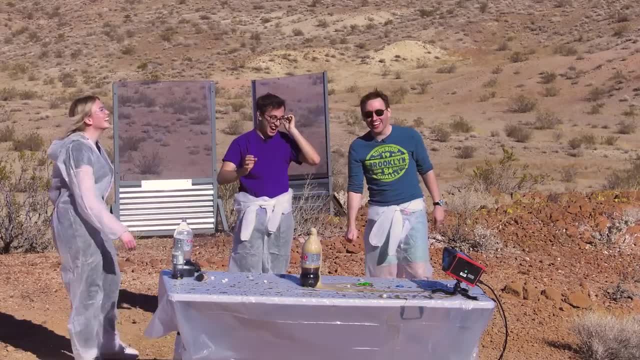 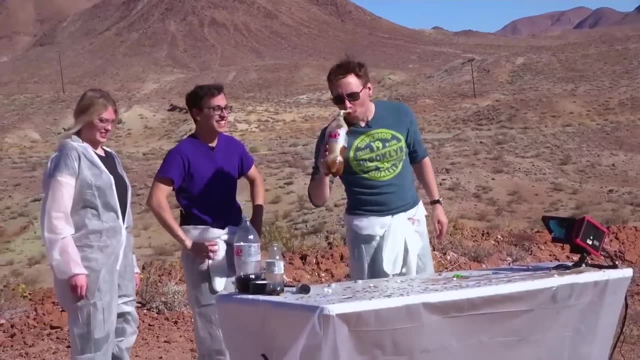 Nice. What is happening in there? Oh, Hey, Yeah, Yeah. Yeah, That went well. That was exactly as planned, actually. You know, that's the very basic, Typical explosion of Coke and Mentos. right, Look, I can do it too. 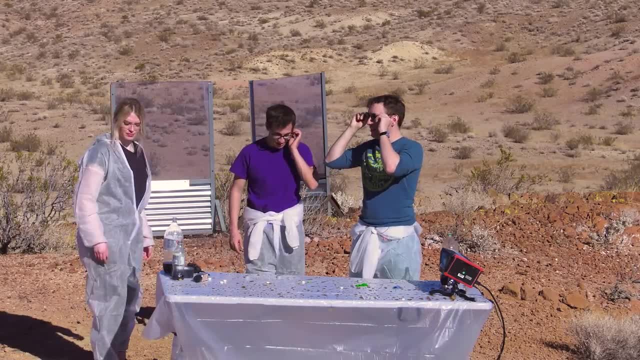 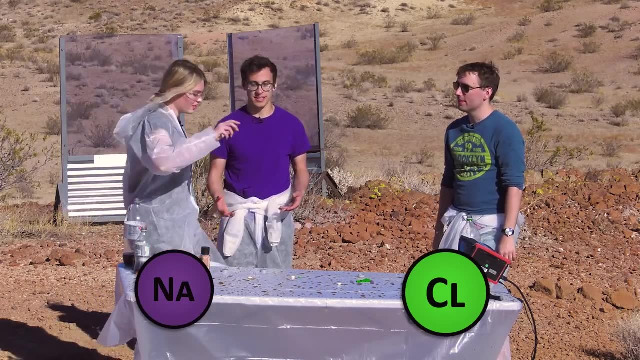 Science. That was the first experiment, So the next one. let me explain to you why this table salt right here can be deadly Table salt is NaCl. right, It's sodium and chlorine together, or NaCl, as scientists say, But separately. chlorine gas will kill you if you breathe it in. 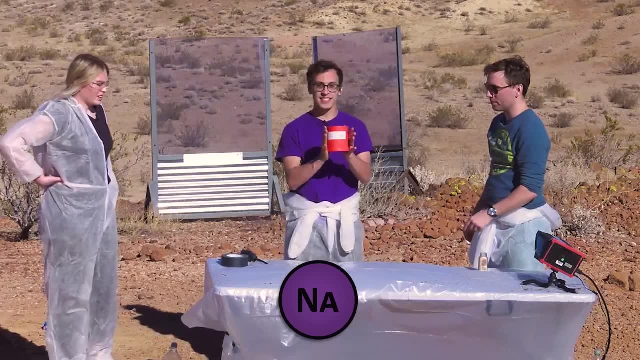 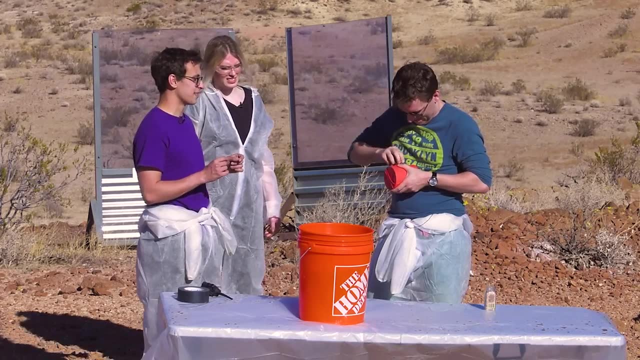 We actually have the other half of it. We have pure sodium. This is pure sodium metal and it reacts violently with water. If I just peel off the warning label that says NaCl, you're not. Yeah, yeah, That's all you need If you tear off the warning label. 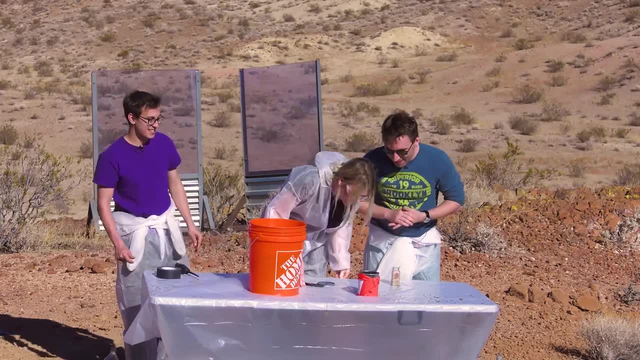 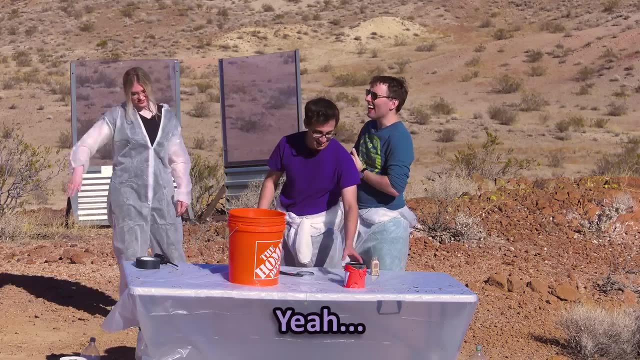 it's no longer dangerous. Yeah, that's what I've heard. That's what Bill Nye does. What's it sitting in? So what it's sitting in is oil. Oil dislikes water Dislikes water. Yeah, because of that bad blood they have between. 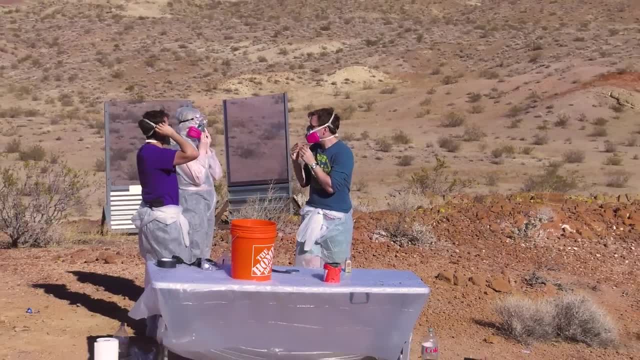 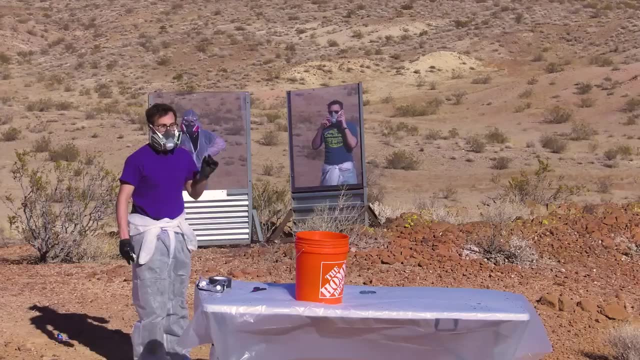 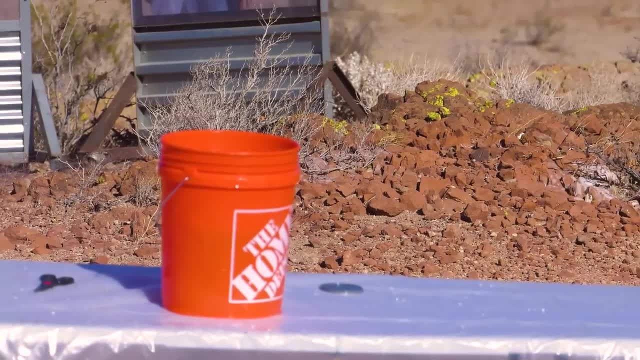 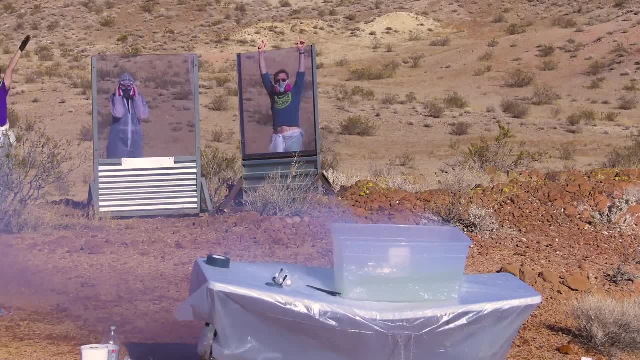 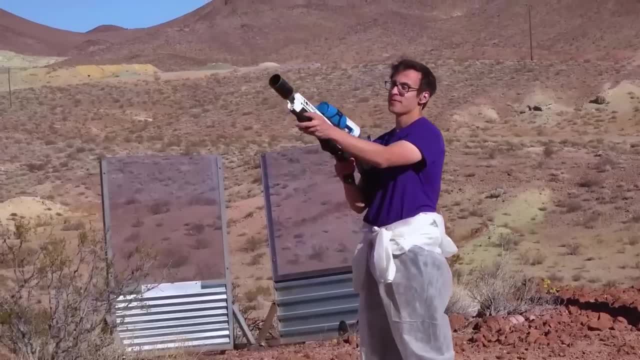 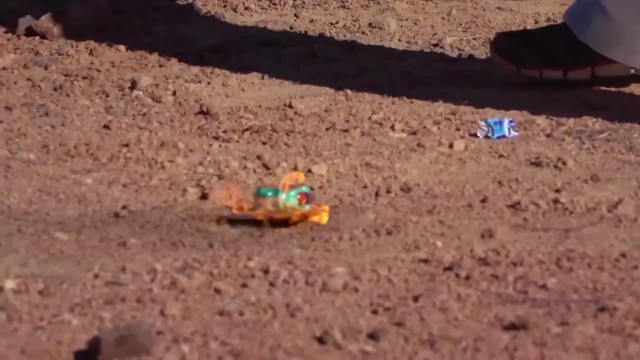 This is busted. You guys want to do something bigger? I don't know. now, Oh shoot Dude, the plastic is melting. Oh my God, This is a good segment for our sponsor, NordVPN. If you are browsing the internet right now, 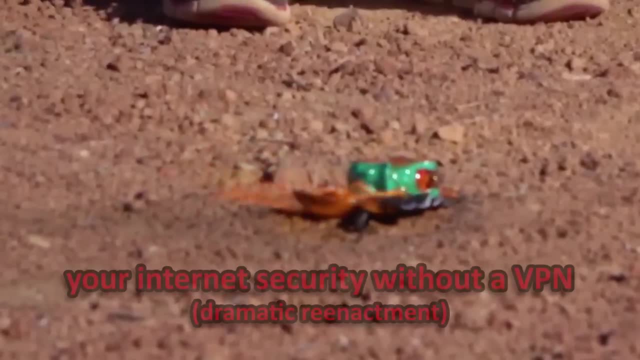 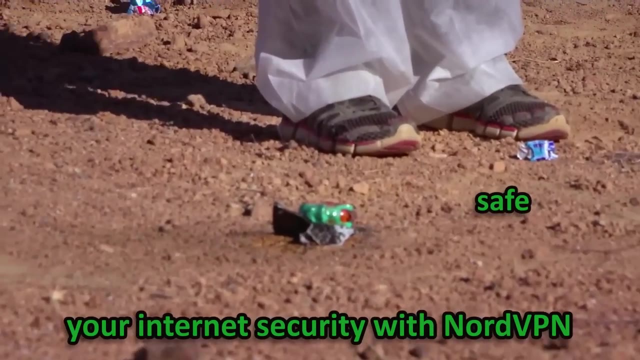 and you are not having a VPN on currently. what are you doing? You need NordVPN. Your internet security is just like this car and you need something to protect you. It can also do streaming services. Let's say you want to watch a show. 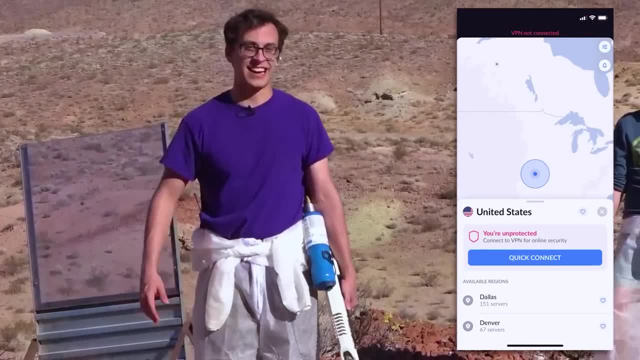 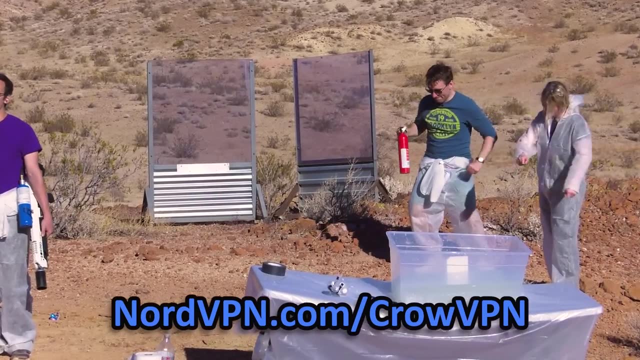 and it's not in your country. NordVPN is the easiest and fastest VPN that you can use. All you need to do is go to nordvpncom, slash crowvpn and you'll be safe. Not like that car, It's a little toasty. 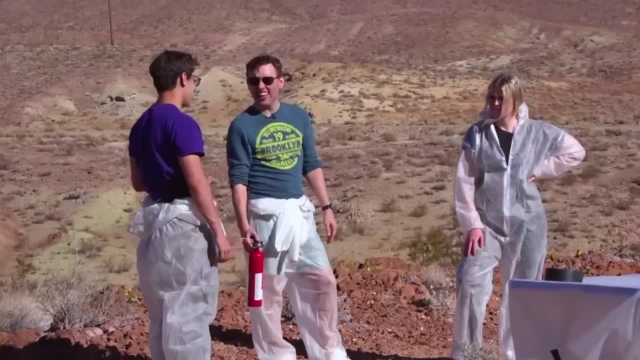 I'll save us. Oh, you have to pull the pin. Little known fact. Did you not know how to use the fire extinguisher? You picked the right guy for the job. I gave you the fire extinguisher: Toss it down like a grenade. 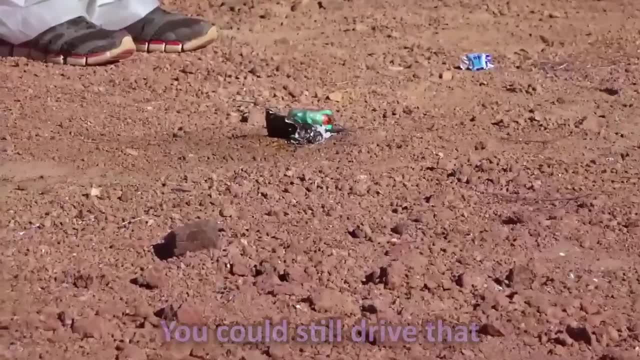 So was that big at all? Really, You didn't even touch the car. Yeah, the car's fine, You can still drive that. So what if I told you we have an actual car? All right, Your shirt is so funny. 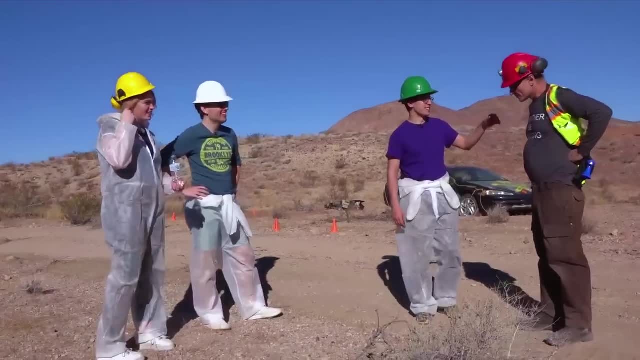 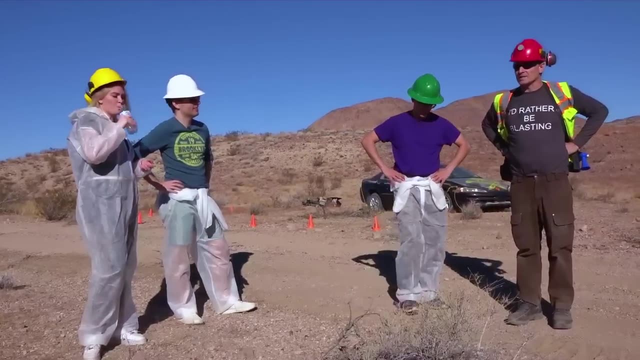 I'd rather be blasted. What is your name and what do you do for the general audience? I am John Norman and I'm a licensed blaster and usually I do rocks and like small demolition and different things like that, and I just wrote a paper on rescue blasting. 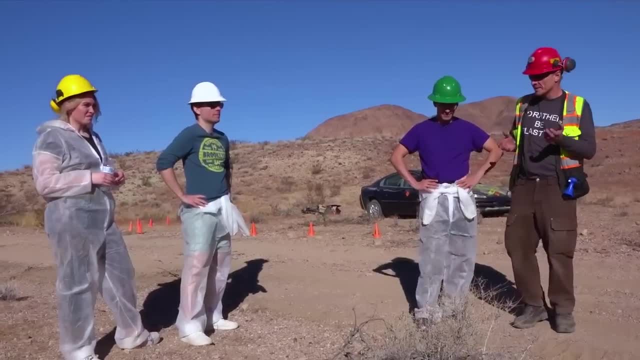 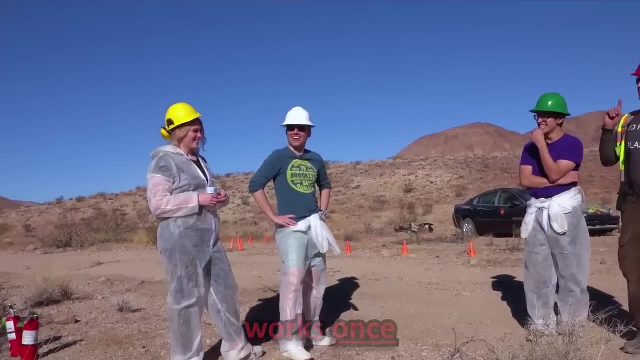 Wow, Oh cool. What does rescue blasting entail? Basically, it's the idea that you can use explosives to remove rock and debris to free a trapped person. What about from my depression? That works. That's like a whole other field of study. 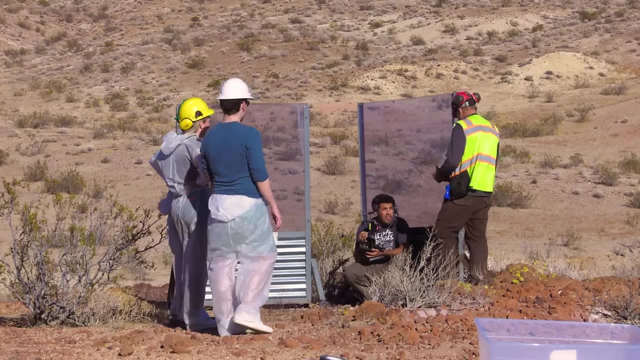 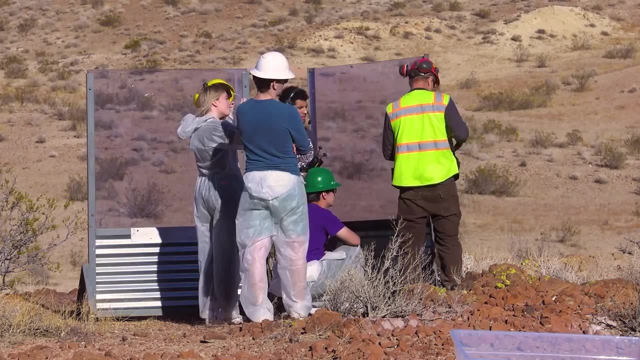 Hey, I mean, are we ready to prime this? Yeah, We are going to hook this thing up. You give a countdown and you say fire in the hole, and then it blows up. We're also going to give a warning with this air horn. 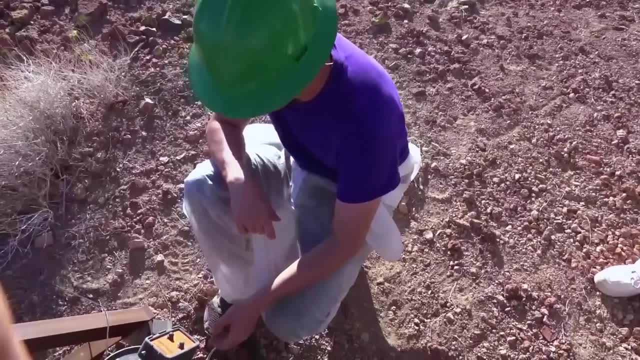 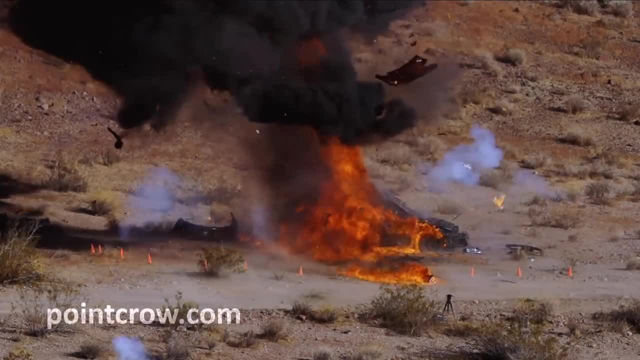 Ready, Jesus. All right, go ahead. All right, here we go. Three, two, one Fire in the hole. Oh, Oh, Oh, Oh, my God, The door, My God, That was like Yeah. 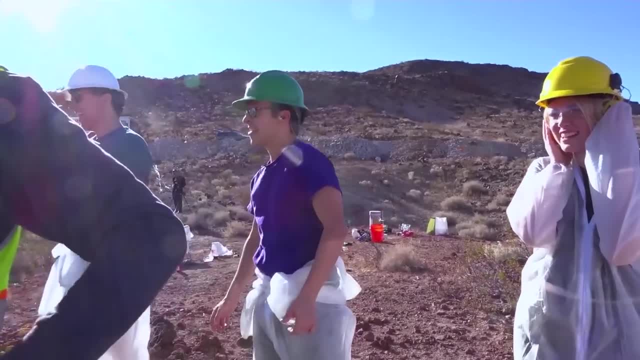 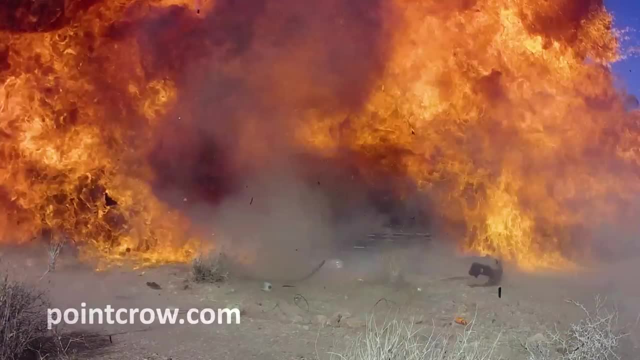 That was. That was crazy. That was so nuts. Was that what you expected? No, I thought it was going to be less. That's crazy. And, guys, that was only about one pound of high explosives total that went off. Can I go see it? 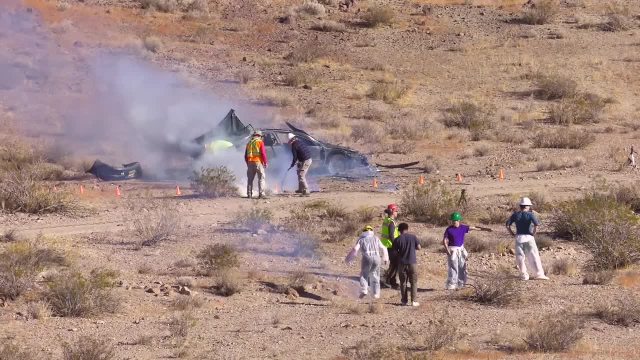 That is so crazy. There is no car left, The door like landed, like over here. Oh, you want to go find the door? Oh, no, You know what that was. That was the roof. The roof came off. Oh, the roof part. 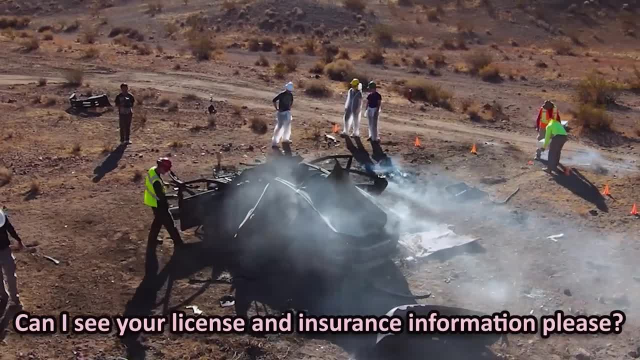 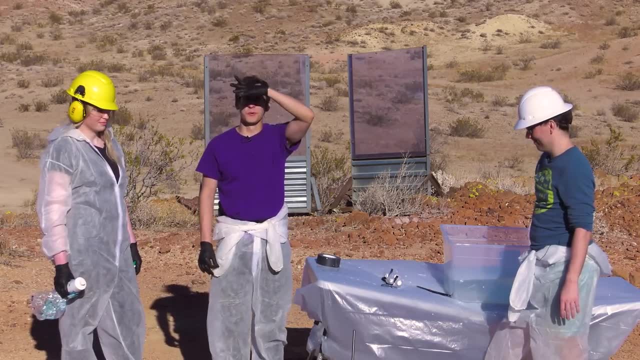 Whoa, That was the dynamite. Yeah, Hey, can I? Can I see your license and insurance information please? All right, Let's head back up. So there's this thing called elephant's toothpaste, And it is one of the coolest reactions. 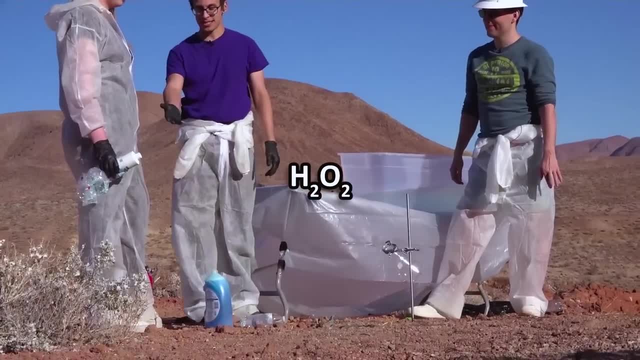 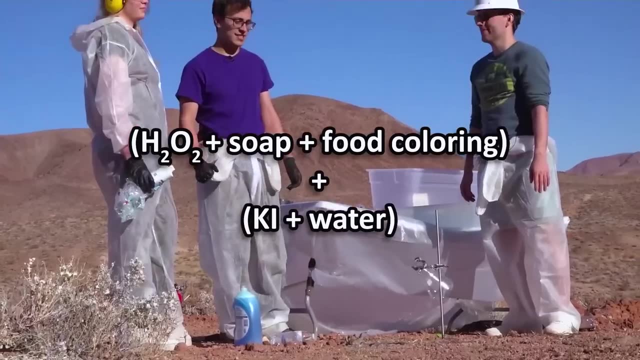 in my opinion of chemistry. Basically what it is is hydrogen peroxide mixed with soap and food coloring. Then, when you put potassium iodide in it with water, essentially it explodes in a really cool way. All right, So, Cutie, if you would like to do the honors of this. 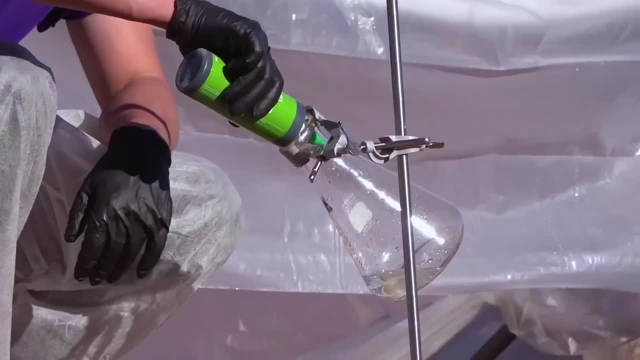 put the hydrogen peroxide into the Erlenmeyer flask. All of it, That was a lot of food coloring. We're going to put a little soap in it too. Beautiful, Look at that. Okay, That is our base solution here. 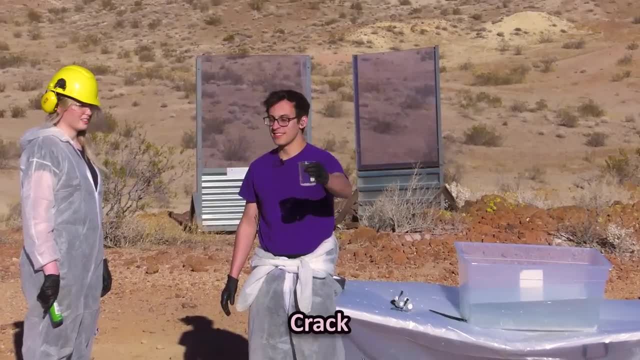 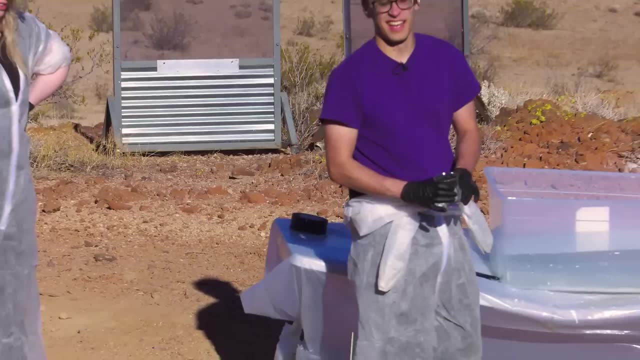 And then this might be a little bit much, but it is potassium iodide And we're going to mix it with water. Perfect, Yeah, I'll mix this around too Awesome. And then this is how the elephant's toothpaste experiment goes. 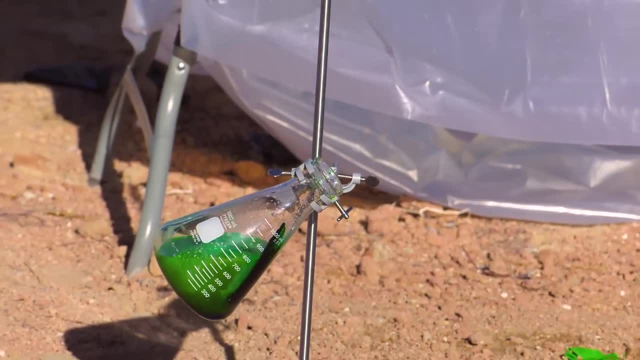 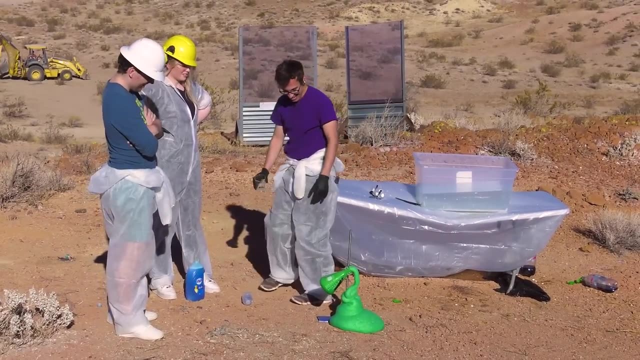 This is going to be a very small one, And there we go, Whoa, Whoa, Yay, So green. And that is the elephant's toothpaste experiment. That looks like boogie-boogie, Is it hot? It is very hot. 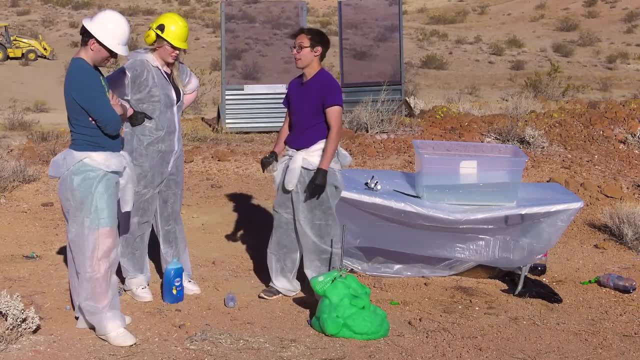 It is an exothermic reaction, So when you put it in, a lot of energy is released in the form of heat. I want to touch it now. Oh Whoa, It's not hot, It's just warm. But let's do something bigger. 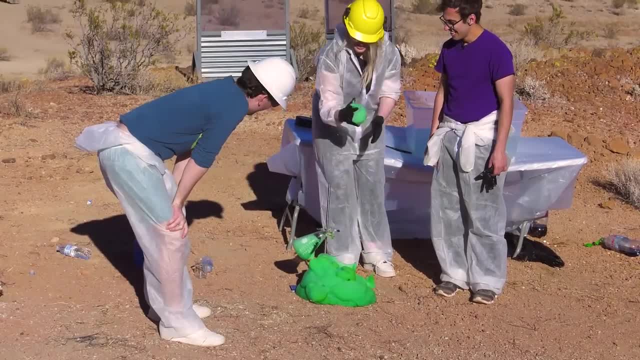 We're going to break the world record for the largest elephant's toothpaste experiment. You want to go check it out? You mean that giant dumpster over there? Yeah, That giant dumpster over there. Yeah, That giant dumpster, That giant dumpster. 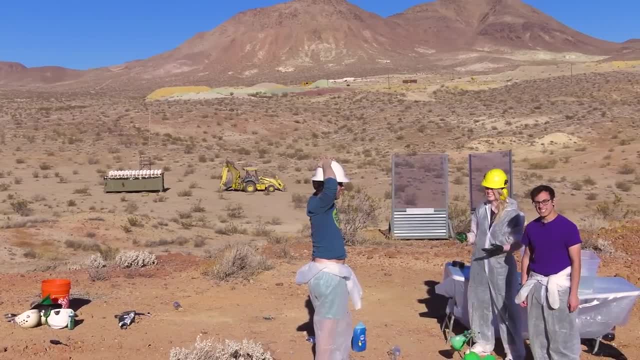 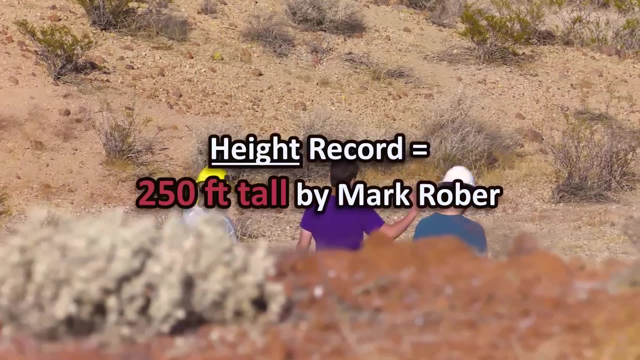 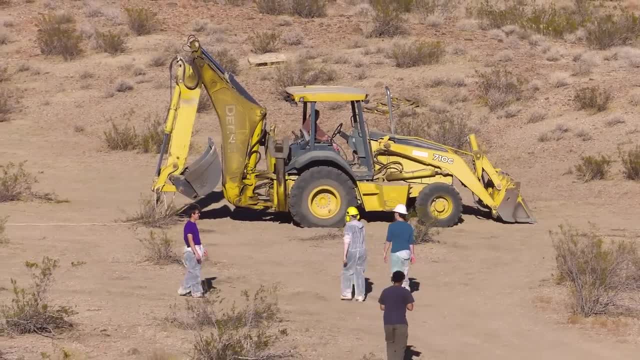 This is going to be crazy. Yeah, you saw how big that one got right. Yeah, how big that one got for that. That was tiny. That was about a little less than 200 milliliters. So what's in here?